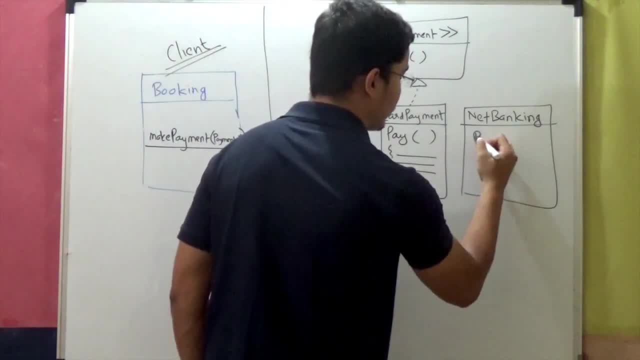 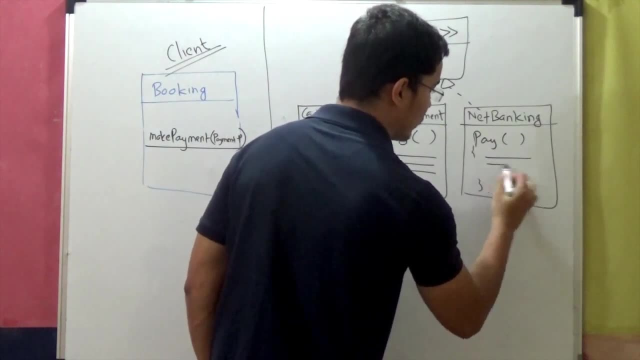 like saving card details and everything. And netbanking will also have its own way of doing payment, So we'll say pay method here. Cash payment will also implement this payment interface And netbanking will have account number, bank name, user ID, something like. 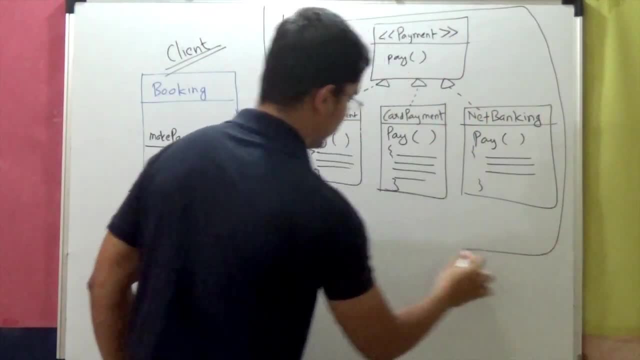 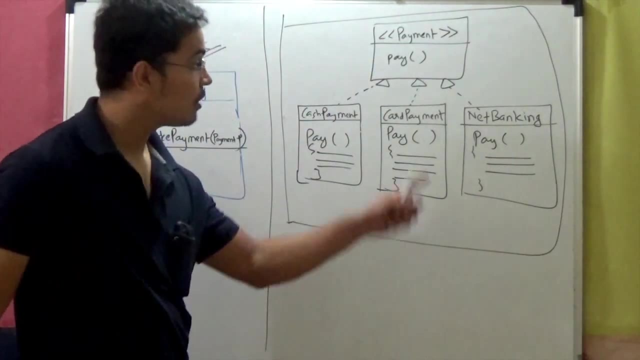 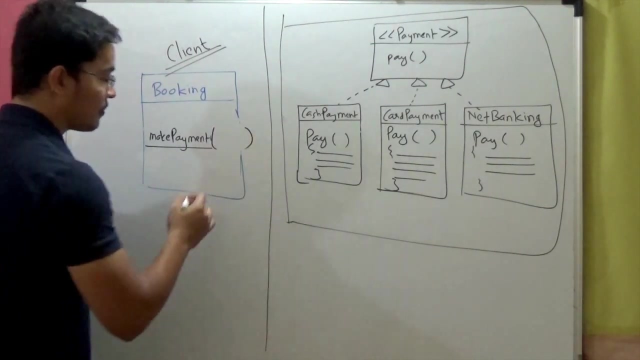 that. So this is a family of algorithms, While each algorithm is encapsulated into classes. Why they are family? Because they are adhering to a standard, that is, payment interface. And now here we will program to supertype, We'll program to interface. So 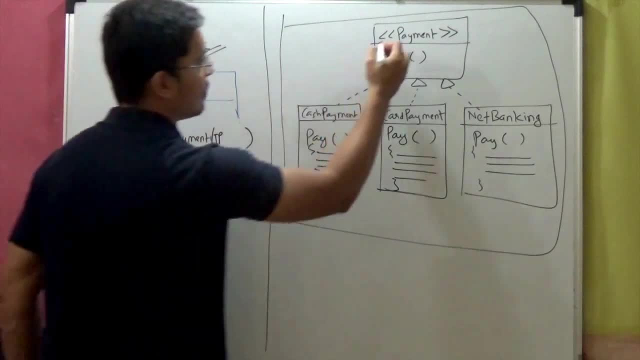 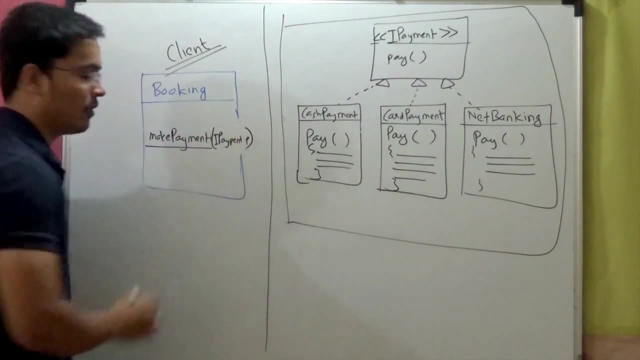 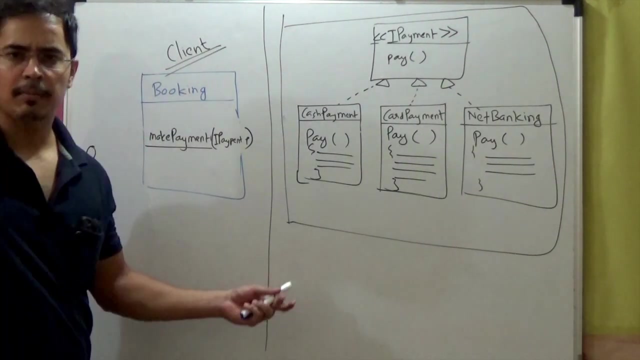 if payment we'll have, let's say, IPayment, We'll call this as IPayment interface And it will require instance of IPaymentP. So let's say user1, who is doing booking wants to do card payment At runtime. he has this option right On his user interface page. 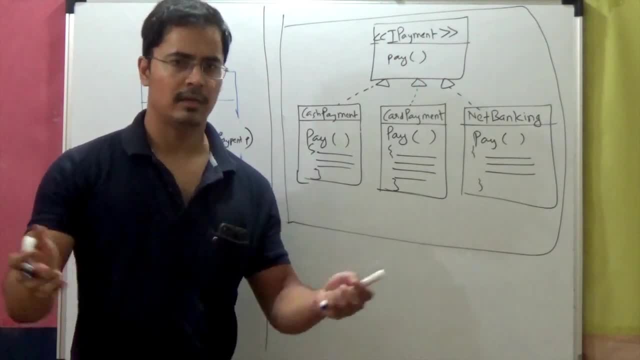 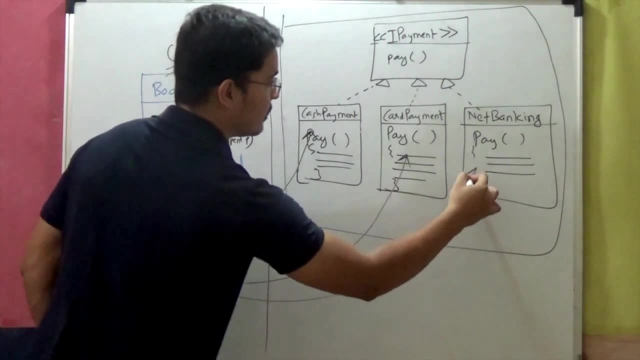 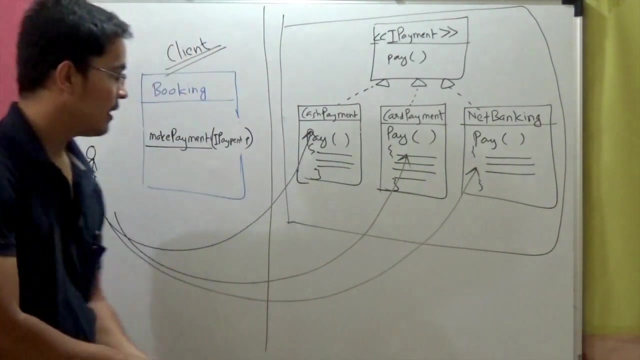 there are options: Card payment, cash payment or netbanking. At runtime he can choose the payment. He can choose cash payment, card payment or netbanking. So there's a flexibility. These algorithms, these behaviors, are interchangeable, right, And they can vary without changing. 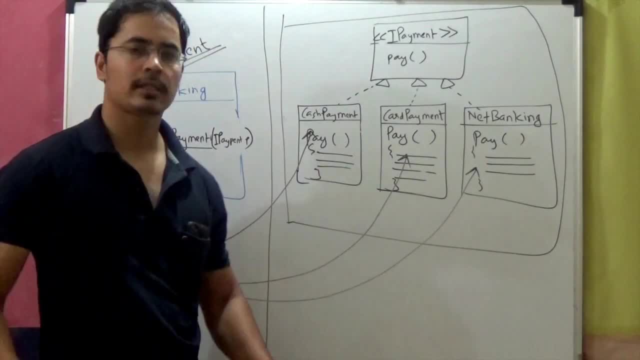 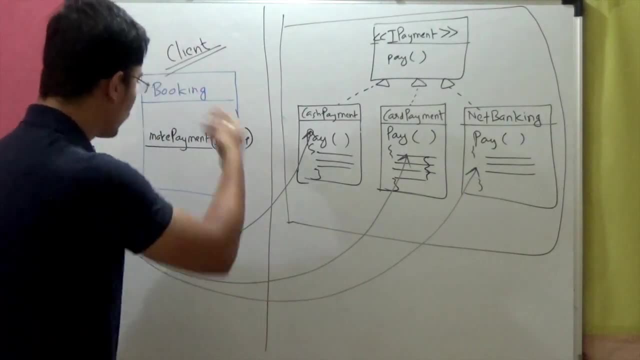 the client. That means tomorrow we want to give discount on card payment only. So we can change the code of. we can reduce the amount here And you don't have to make any change in your client code. You can change netbanking. 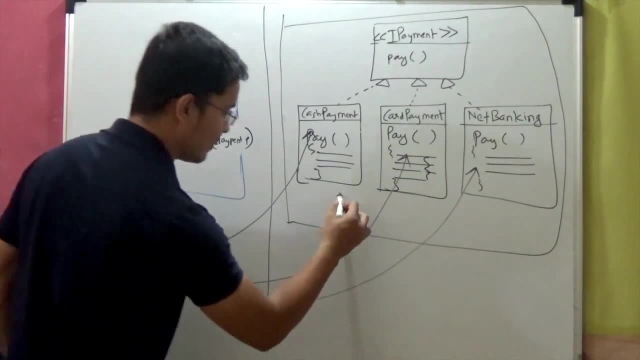 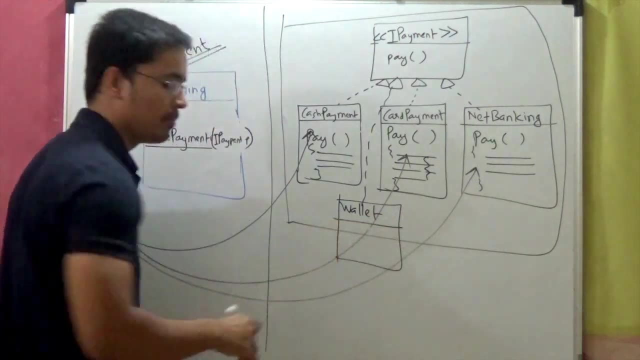 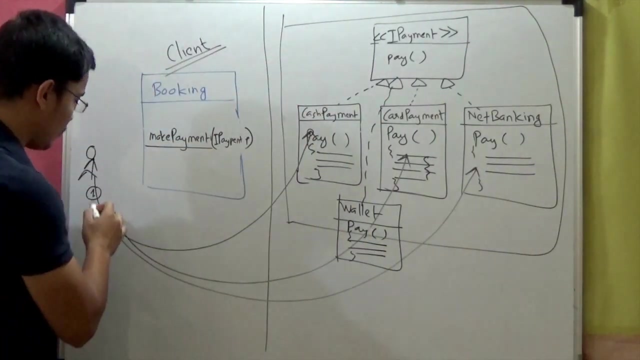 You can give more discount on netbanking. Or tomorrow you can add another new way of payment, Let's say wallet payment based on any wallet system- PayPal or Paytm or free charge right- And it will plug in: User have one more option at runtime, Instead of three. 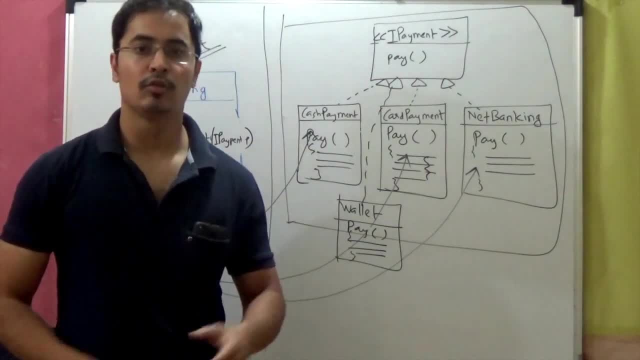 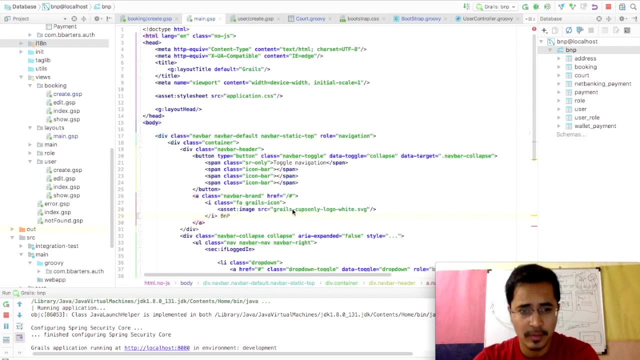 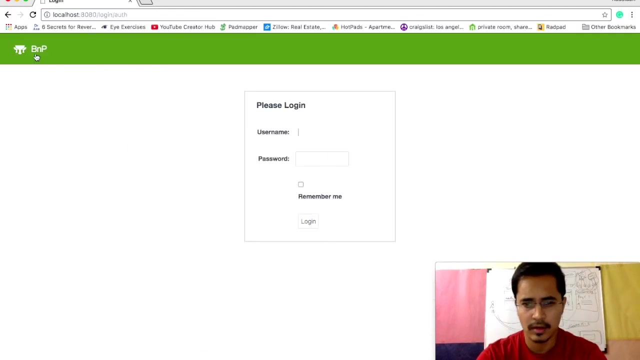 it will have four, And let's implement this strategy pattern solution in using programming examples in our tennis complex application. So let's start. Let's start with our programming implementation of strategy pattern. Let's just first run our tennis complex application Book and play Fancy name. So I've created this one user. 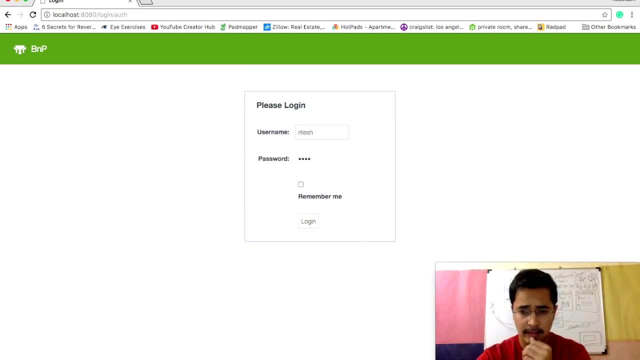 So I'm using this framework called as Grails. It's MVC framework. It uses a language called as Groovy, But this language is very similar to Java. It's a superset of Java, So you will see me using Java classes. 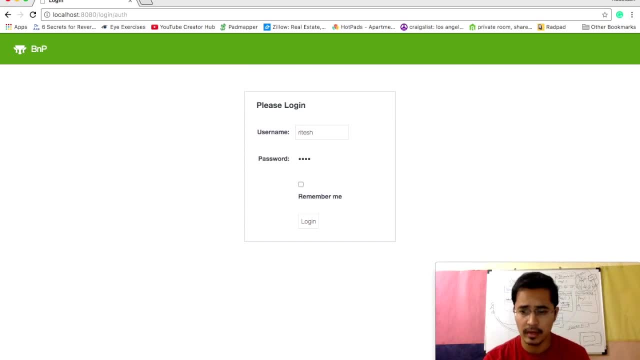 Write Java classes for implementing our design patterns. If you want to know more about the basic fundamentals of how to use this Grails framework, I have put two videos to get started with Grails. You can just check them out. So let's just log in with this user And right. 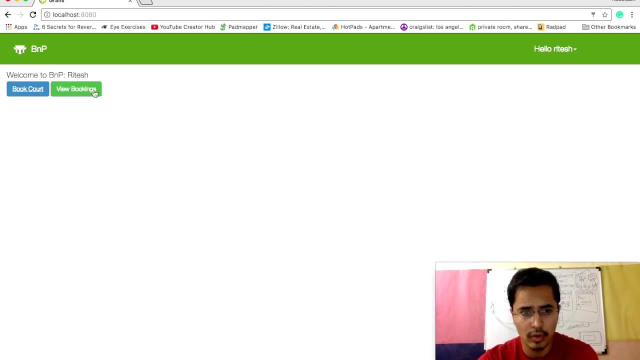 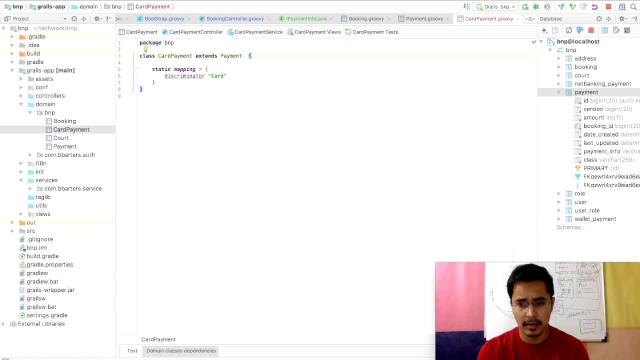 also make sure that we will provide our card payment behavior. so it has to implement our I payment info interface right in our payment model into add a field for storing the payment details. so just an object and that's a payment underscore info. so we'll do that in our card payment class. as I said, we want to. 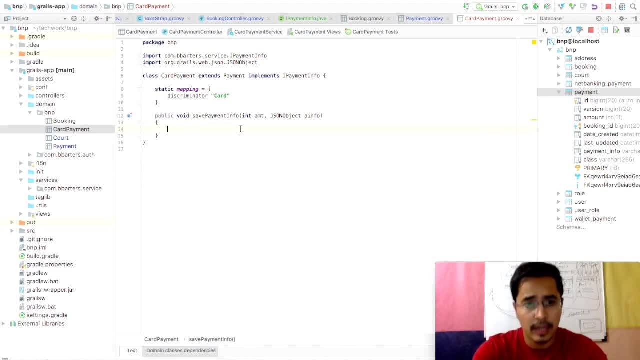 give certain discount on the final amount. so in card payment I want to give 20% discount. so I'll say this: dot amount, the final amount equal to whatever the amount that has been given to us. when the user selects the code and the amount is determined based on code charges, it will pass down here in the form of. 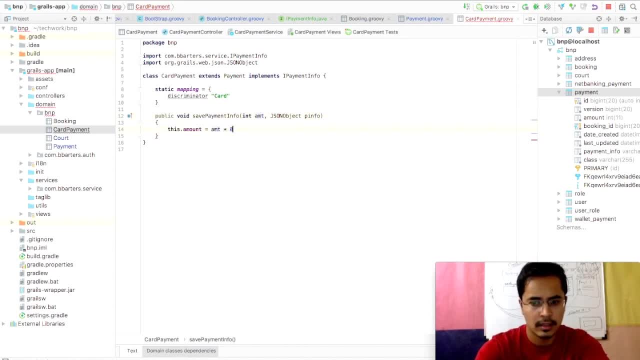 parameter and then say amt star: 0.0, 0.8. so that will be our final amount, that with 20% discount. and then we'll say this dot payment info. equal to this JSON object info: cool, so why it is a JSON, this payment info? because I don't know what kind of information I'm. 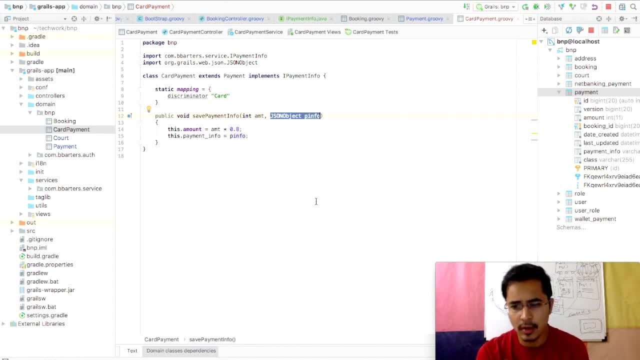 getting. so I don't want to create multiple columns for different kinds of payment info. rather, my idea is: in my payment table I'll have just one column as payment info and it will be a JSON. so it's a flexible arrangement. JSON can have different kinds of fields. there's no restriction upon type of field. so for 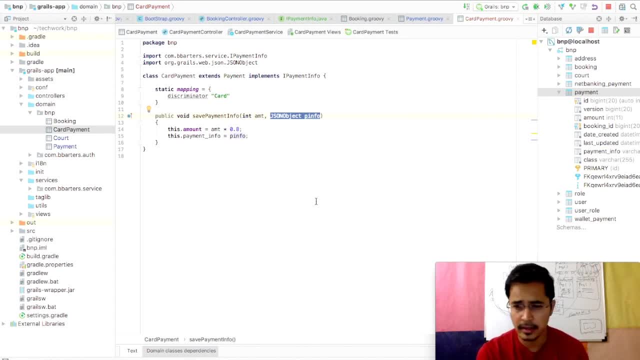 card payment. the JSON will be like card number, card type, bank card issuing bank name, something like that. for net banking it will be bank name, account number and so on and so forth. if you want to store miscellaneous information, which is going to be different for different rows in your table, it's advisable to use the 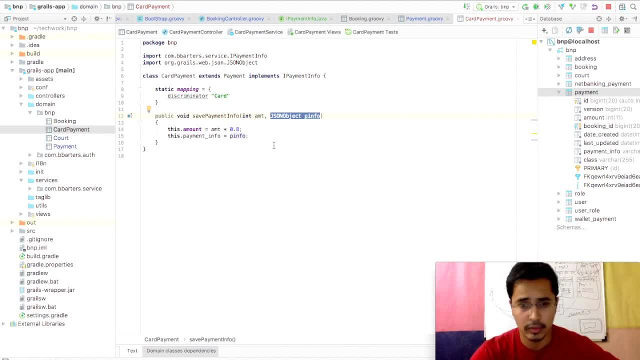 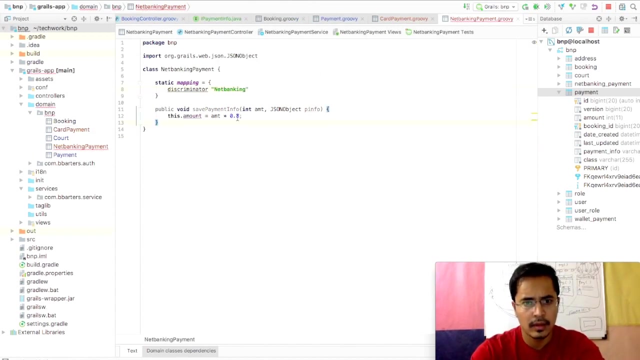 column as JSON, because just one can allow you to do that. so I'm gonna do that. cool. so this is my one behavior. so I need to provide behavior for net banking, wallet and cash payment right, so let's do that. and here the discriminator will be net banking. in net banking, I'll use 15% discount 0.85. this dot payment info. 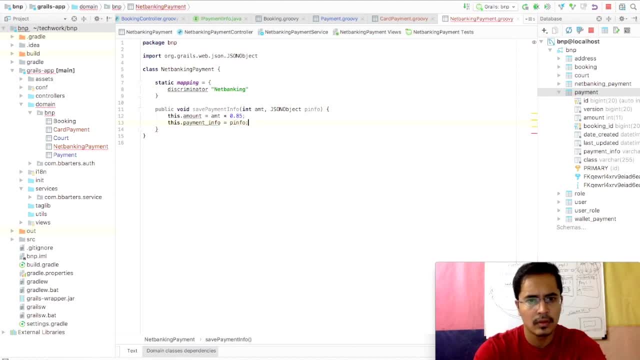 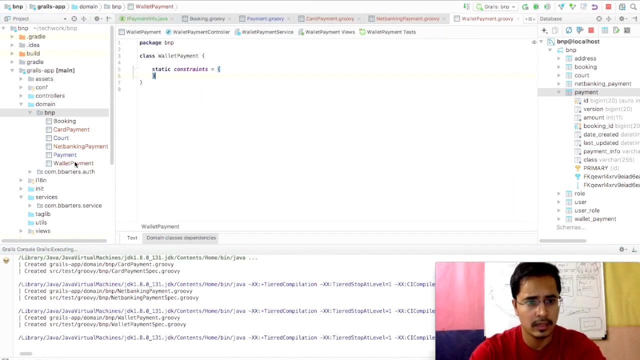 equal to info who. obviously, this net banking payment has to extend the payment and has to implement the I payment info interface right. similarly, we'll create two more, that is, wallet payment and cash payment, right, so I'll quickly write the code for this tube. they will have different discounts all. 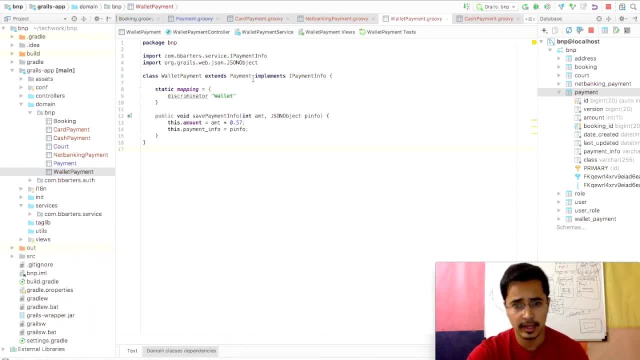 right. so here is my wallet payment plus. again, it implements the I payment info. we are providing implementation for sale payment info method. it has a discount of 25% on the amount of booking and also it will store some payment info in the form of JSON, right. so that's pretty much it. so now, what we have done with this code is that. 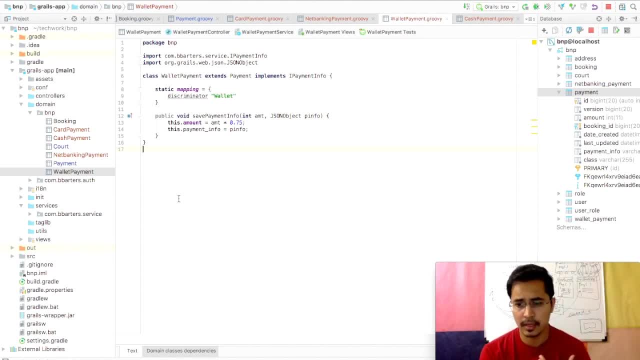 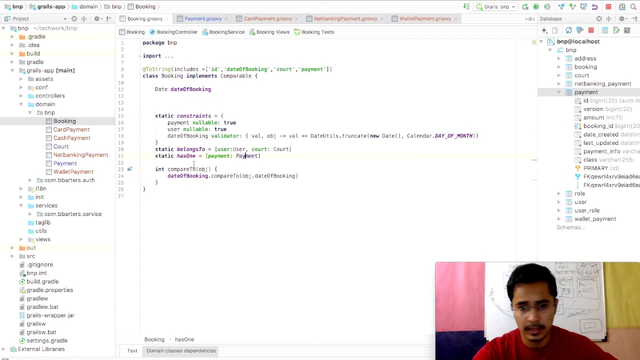 we have formed a family of algorithms. we have encapsulated our different payment behaviors into classes and formed a family because they are all implementing a common standard in the form of I payment info right. so we have created a family of behaviors and our client is our booking class has a super tap instance has one payment and we can. 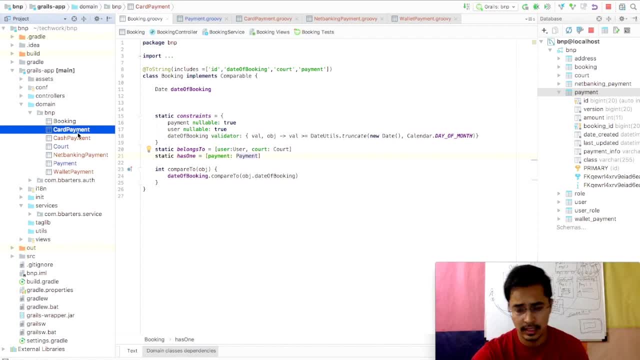 provide any instance of any instance of either card, cash, net banking or wallet, depending on choice of the user. this is our strategy pattern, because client and behaviors, payment behaviors or payment options are so loosely coupled right, because we are programming to a super type here, so runtime user can decide to choose among. 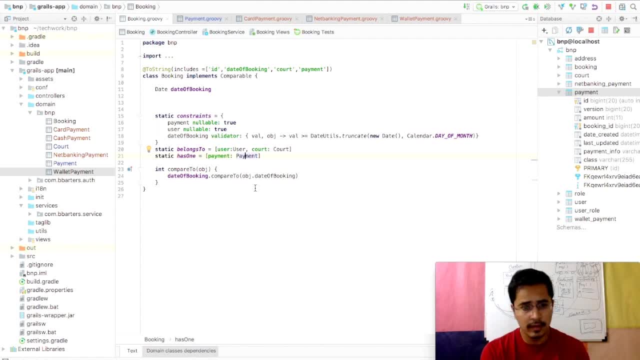 card payment, cash payment, net banking or wallet and will create appropriate object and pass it on and assign that object as a payment option for that particular booking. they are loosely coupled. so fantastic. going forward, tomorrow we can make changes in the discount scheme. we can change the discount percentages, we can remove the discount or we can even add a new. 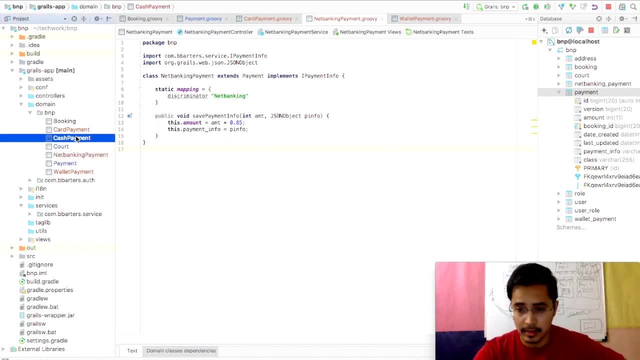 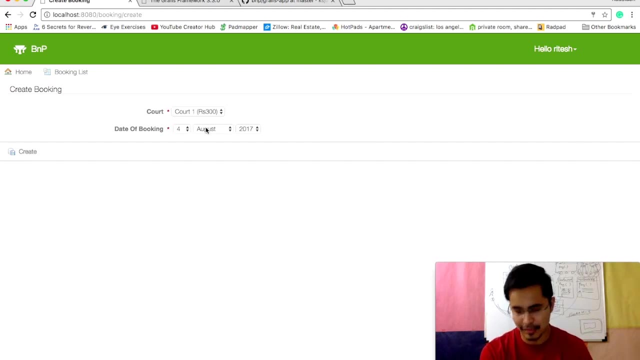 payment method like barter payment or something like that, and without disturbing our booking class. awesome, so this code looks good, so create booking is pretty straightforward. this UI was meant for cash payment only, so I have to make the necessary changes for user to be able to decide. 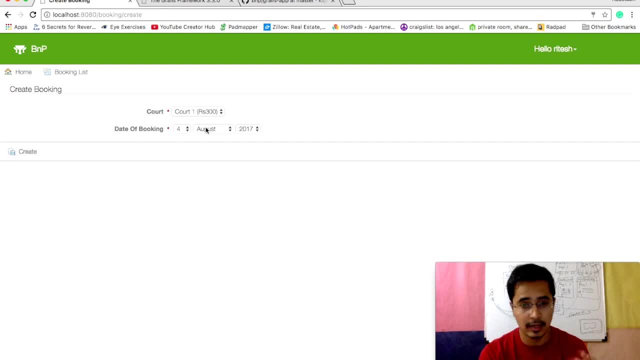 run time, which kind of payment he or she wants to make, right? so I'll make those changes in UI and slight adjustments in my controller and that will be it. so let's do that. so we are ready with all the changes in our views and controllers, right? whatever that it was needed. so I'll just log in again and okay, so I 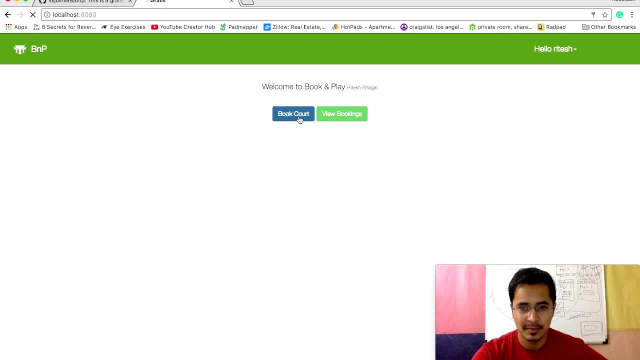 will see if I can actually get it done. my account it's a little bit slow, so let's put it back in the account. alright, so I will do it in my account. so if I release it right now and let's see if it works, like this guy, easy as is, but I 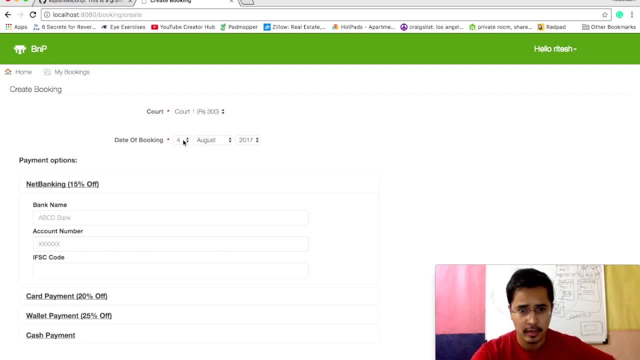 will go to my account window. I will click on my account. so let's hit here now and it will check whether it is already in the account or not. so I will click, click on my account now, let's you can see that here. let's have a look now. 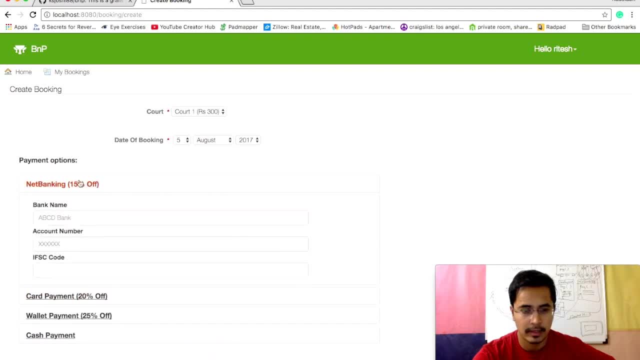 let me click on my account and let me see what else I can do. okay, so I'll check. we are net banking, right? okay? so let's just do card payment. so i'll say issuing bank name as bank of america. all right, card numbers? okay, one, two, three, four, five, cvb- oh my god. six, seven, eight. 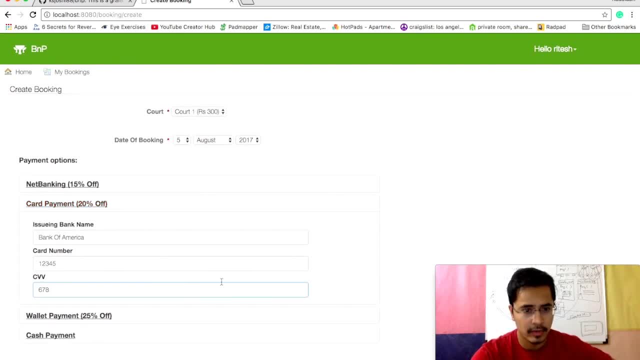 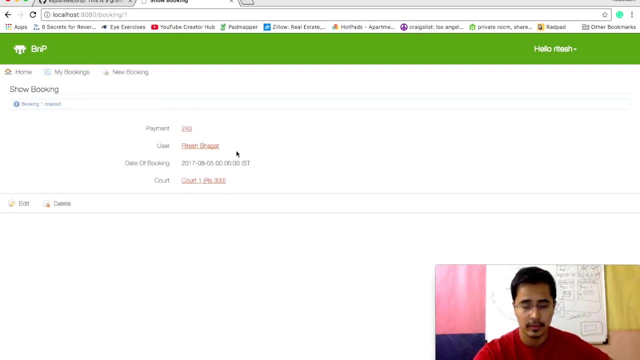 awesome. so that's 300 right and 20 off. so i'll say: create booking, okay, awesome. so booking is done and total payment was 240. is that okay? yeah, i think so. so i got 20 off on my card payment. let's see the database entry. what has been the database? 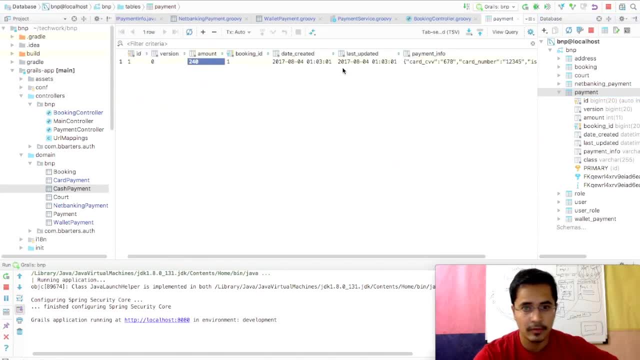 so i'll go in database. so there's one payment of 240 and look at this payment info, json that i was talking about card, cvb, card number and issuing bank name is there in one column right and i told you single table inheritance in this payment table entry, the class is card, it's a. 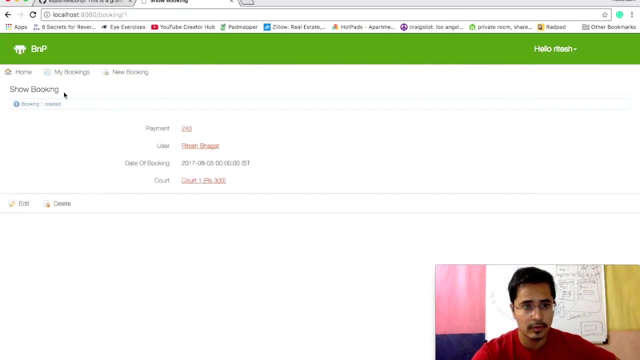 card payment. it's indicator that it's a card payment. let's go and do one more payment. so let's go home and let's say the quote and i'll book for 9th of august. i'll make quote four. cheaper quote. i'll say: this time i'll say net banking- yeah, why not? i'll say: an account number is. 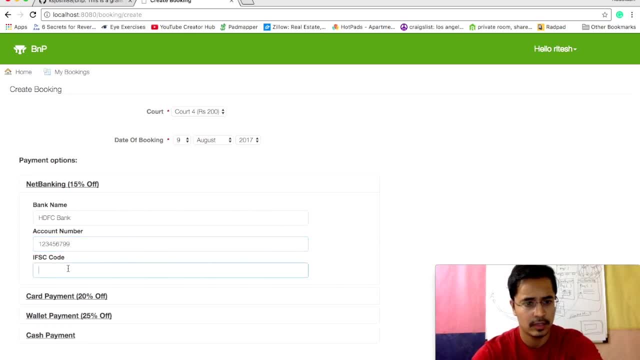 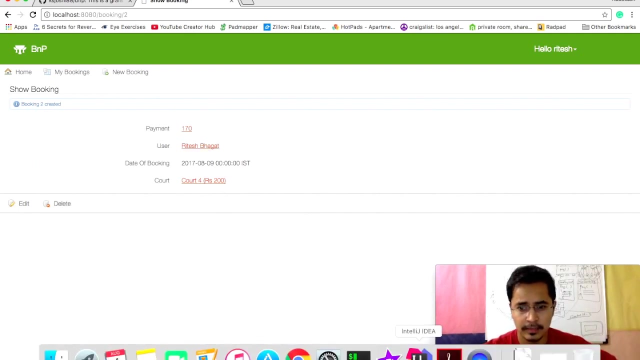 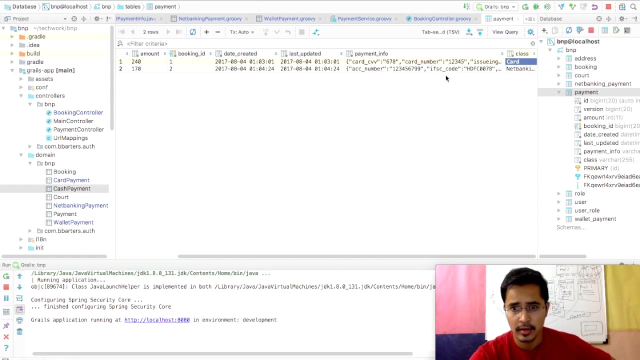 14, two, three, four, five, six, seven, eight, nine. pretty good ipc code: atfc: zero, zero, zero, seven, eight, okay, and i'll say create booking, so 200 and 15 off, so 170, awesome, nice. and let's go and uh, check this payment entry now. so the payment information is there: account number, ipc code and 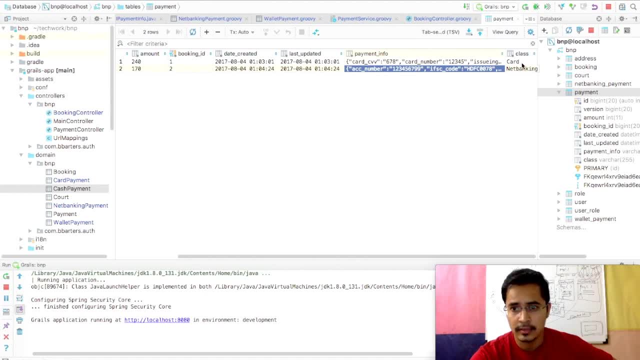 bank name and you can see the class column has the entry of net banking right now. so this is single table inheritance. we are creating the objects of net banking, payment card payment and they're all being stored inside our payment table in our database, right, because they are all inheriting the payment model, awesome. so i want to. 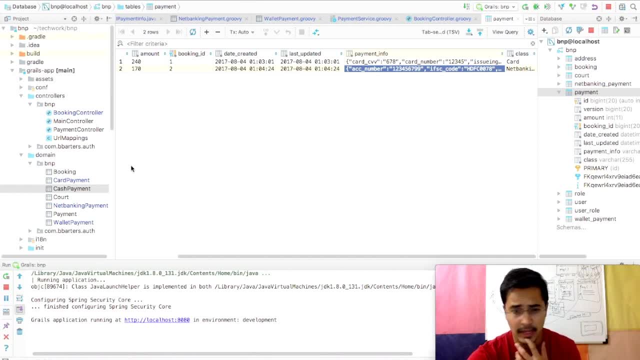 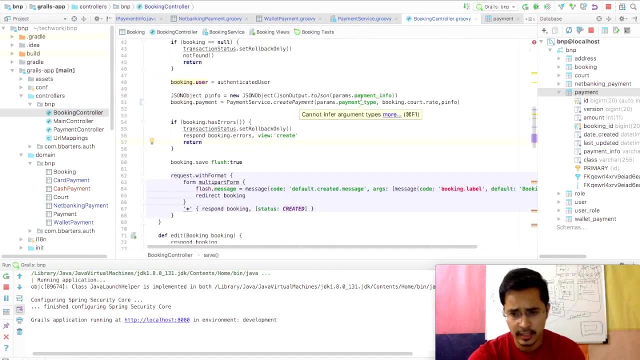 just show you what i did behind the scene in my controller: logic of it, right. so in my booking controller, in the save method. okay, i received the form, the html form, through my parents method that is accessible in grails, to get the parents submitted in the form and i i had always named all my parents as payment info, right, so i converted. 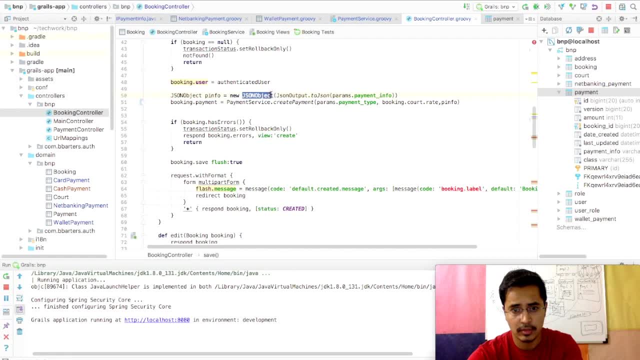 them into json json object because you remember my data type in my payment model for a payment info was json object, so i converted him into this. an object. booking has a payment. you remember that booking has a in requires us instance of payment. payment is our super class, so i need that payment. 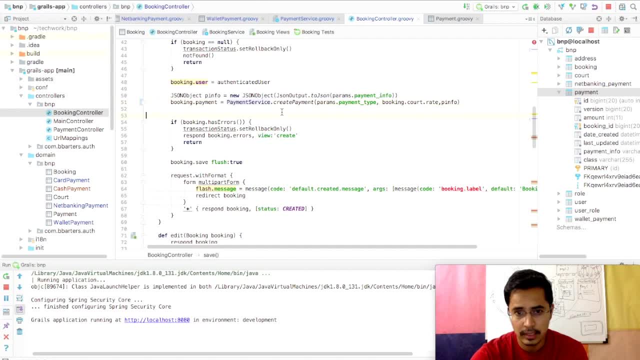 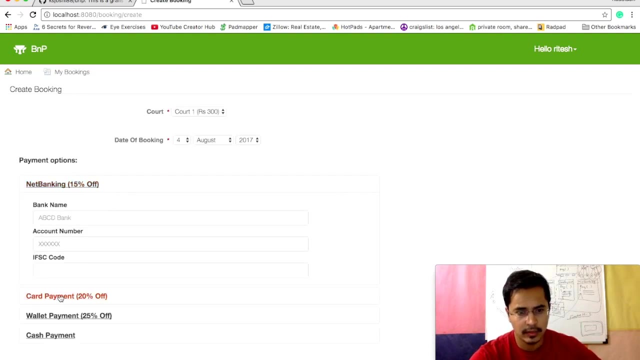 instance, right. so i create this service, payment service, and it has a method, static method, called as create payment. so i'm passing on the payment type parameter which i'm getting from my form, html form. so payment type will depend on which, which payment type i'm choosing here. 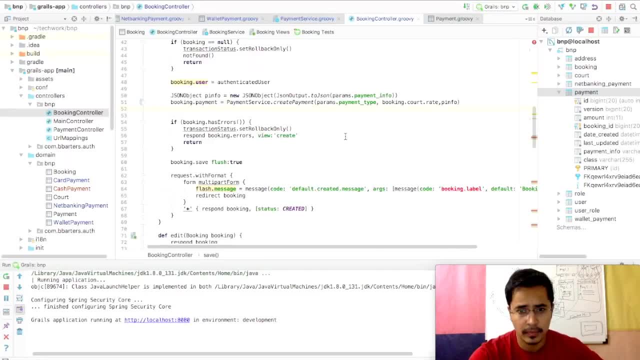 so that will set the payment type. it's a hidden field in my form, right, that payment type, because that will help me create the instance of specific type of behavior: card payment, cash payment or something. and then i'm passing which code he has selected, right? so the code, the rate of the 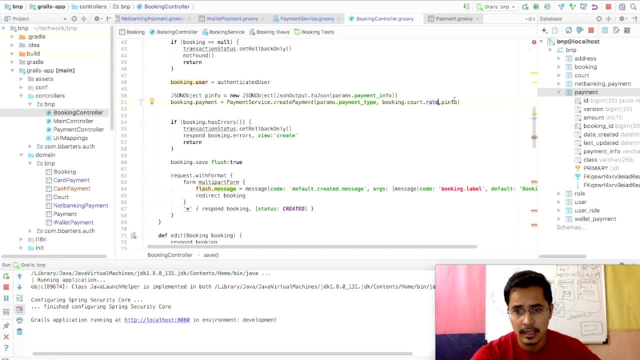 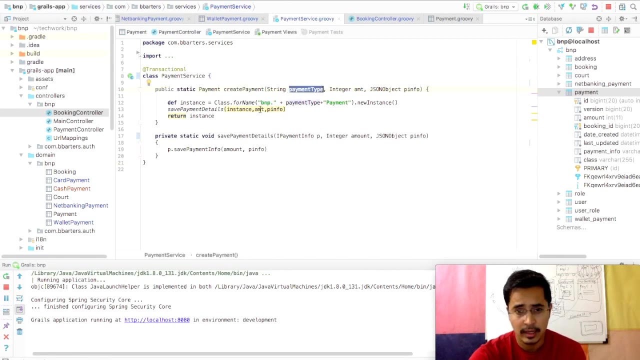 code which will be my amount, initial amount and then p info, is my json that i created from the html form for different kinds of payments in this create payment method. so i'm getting that payment type string from the html form right and using it to create instance. so you can create instance from a string name. you can create class.